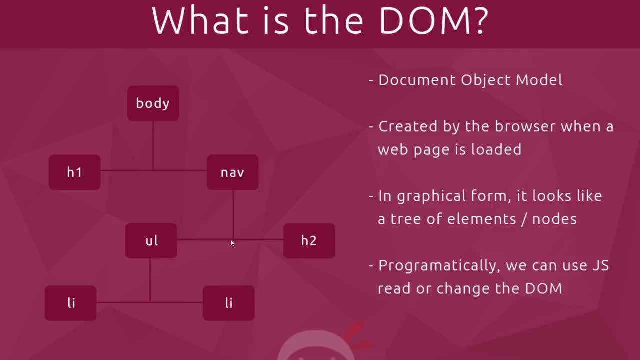 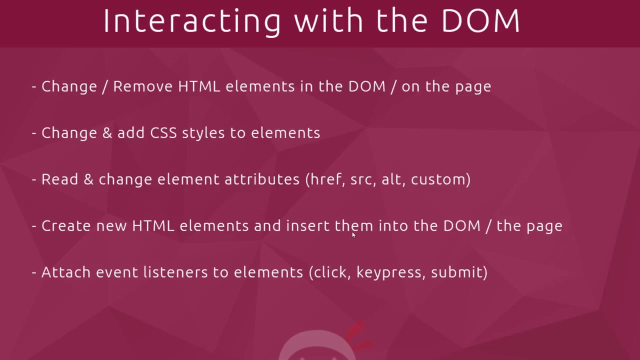 have pairing elements at the top And children elements nested beneath those And, programmatically, what this model allows us to do in JavaScript is interact with this tree, this DOM, and do things with it, And there's loads of different things we can do with it, So some of them are these things here We can change or remove. 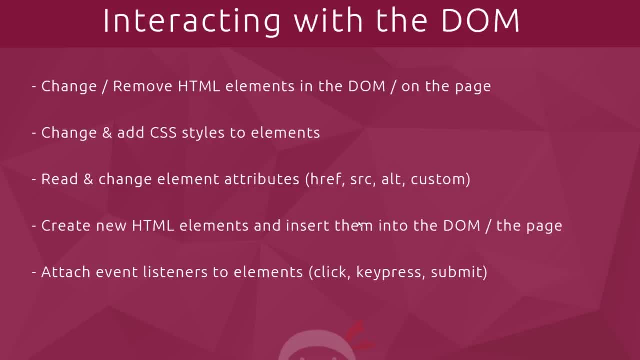 HTML elements in the DOM or on the page, So we could reach in and remove an element if we like to, Or we could change and add CSS styles to these elements via the DOM. We can also read and change element attributes, and by that I mean things like the href attribute on anchor tags or 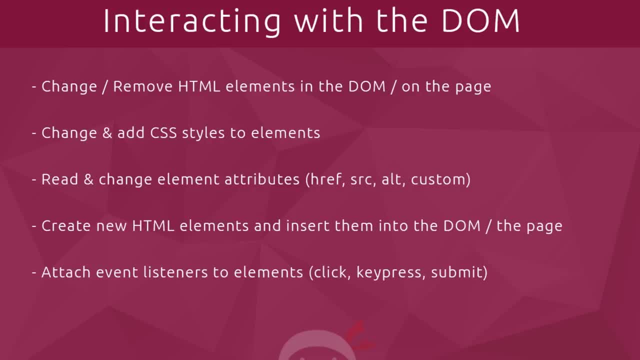 the source attribute on image tags or alt attributes or any kind of custom attribute you may have on your HTML elements. We can also create new HTML elements and insert them into the DOM or the page via JavaScript, And we can attach event listeners to different elements, things like click events. 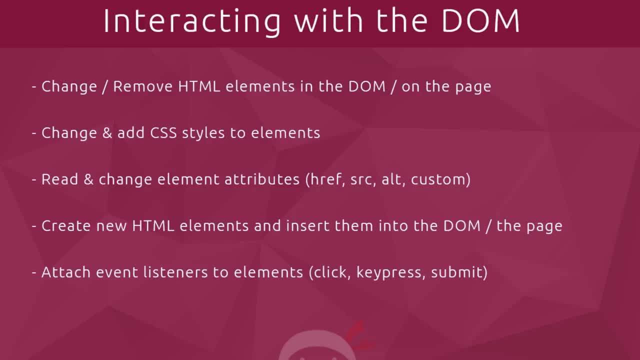 keypress events, submit events and react to those as well in JavaScript. So we're going to be covering all of those elements. So we're going to be covering all of them and we're going to be of this in this series, and you might be sitting there thinking at the minute. well, you know what? 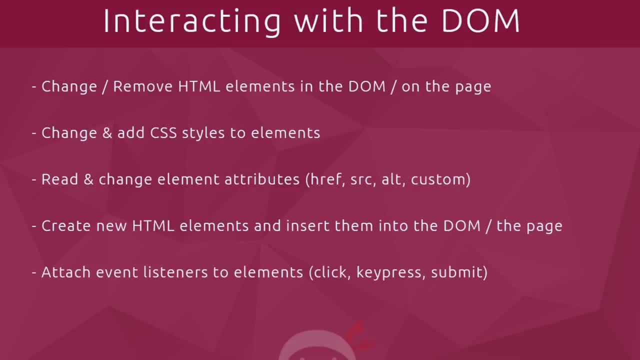 i can actually already do all of this. all i need to do is grab jQuery and i can do all of this really simply with that. and yeah, okay, you probably could do, but i wouldn't recommend it in a lot of cases. i know a lot of developers which just use jQuery all the time only for the DOM, and i think 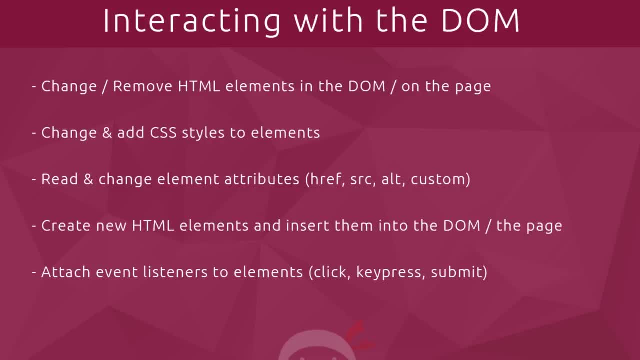 that's kind of overkill, and you can do everything you can do in jQuery just using vanilla javascript, and that's what i'm going to teach you in this series. nothing to do with jQuery. it's all going to be about javascript and how we can reach in and interact with this DOM using only pure javascript. 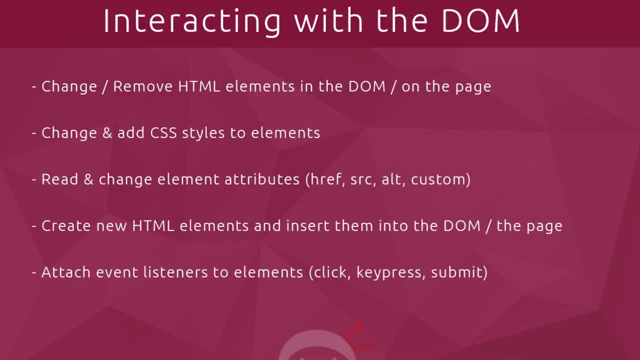 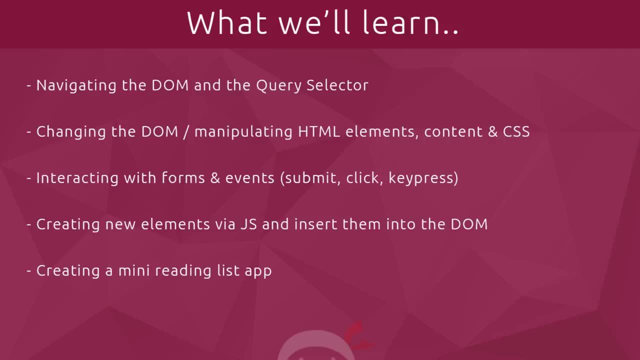 and i think that's much more fun and it's going to make it a much more rounded javascript developer as well. so this is everything we're going to be covering. the first few lessons of the series are going to be focusing on how we can navigate the DOM, go up and down it, traverse it, if you like, from. 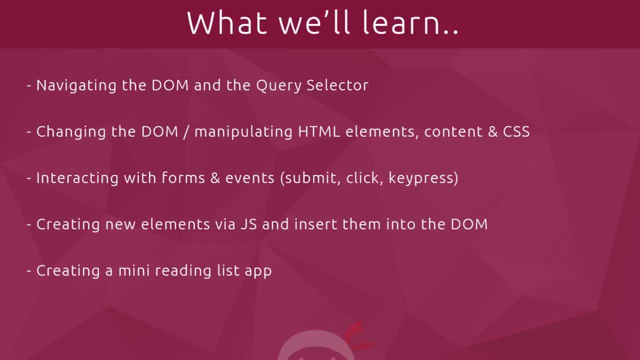 parents, a child, that kind of thing, and we're going to look at the query selector, which is very much like the query selector, which is very much like the query selector, which is very much like the query selector in jQuery. not much difference there. we're also going to take a look at how we 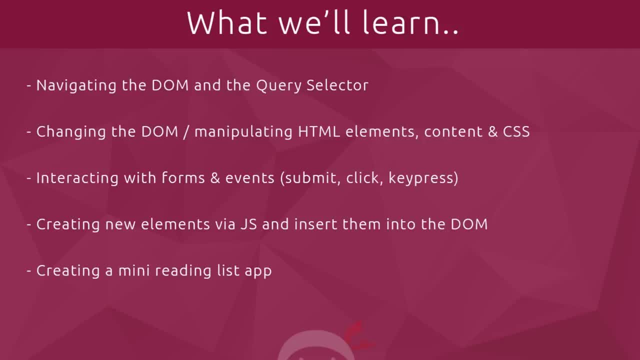 can change the DOM and manipulate these different html elements inside of it and the content within it, as well as the styles as well the css. we're also going to look at interacting with forms and events, things like submit events, click events, key press events, all that kind of jazz, and then 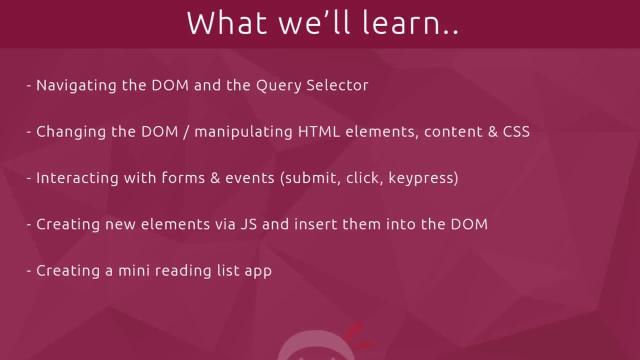 we're going to start creating new elements via javascript and insert them directly into the DOM in different places wherever we like, which is really cool. and, along the way, we're going to be creating this kind of mini reading list app, which I'm going to show you in a second. okay, so. 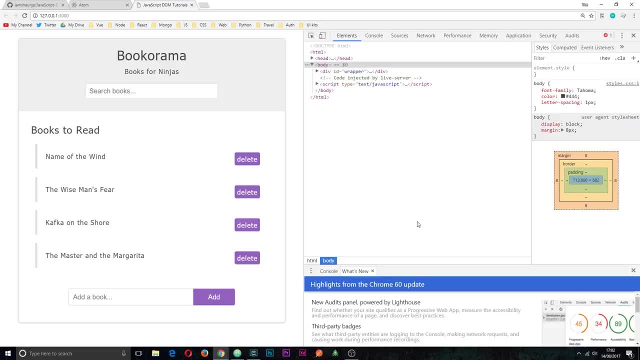 this is the basic application we're going to be creating throughout this series, and I know I'm not going to win any css awards for this, but that's not what this course is all about. we're going to be looking at how we can interact with the different web elements here to do things like 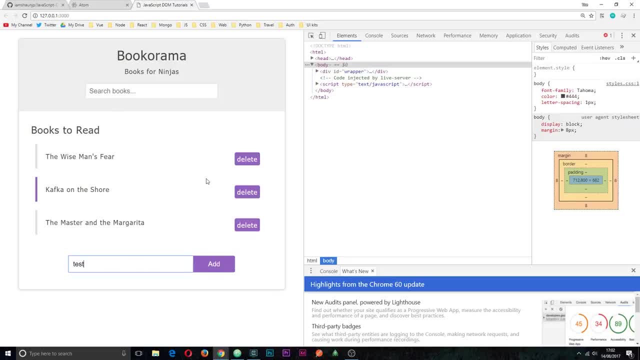 delete books, search for books or even add new books like so. so that's what this series is all going to be about, and we're going to be creating this app as we go along. now I'm going to be using the, the atom text editor as well, which is completely free and really cool, so you can download that at. 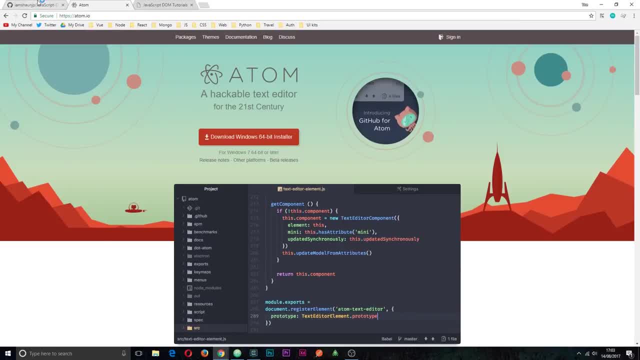 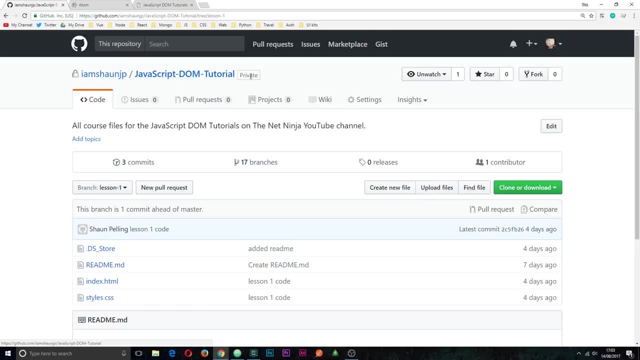 atomio. the link is going to be down below. I am also going to be giving you all the course files for the whole of this series, so every lesson is going to have its own branch on this github repo to be down below. so if you want to check out the code for lesson 10, for example, just select the. 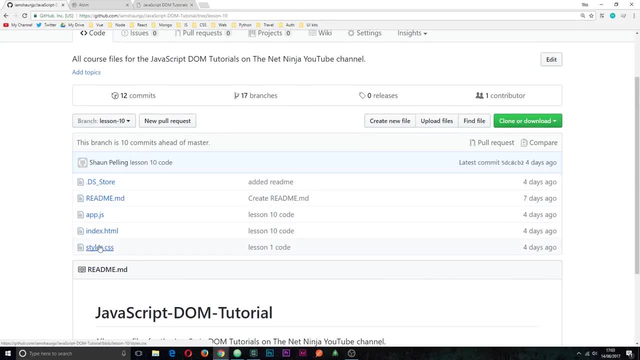 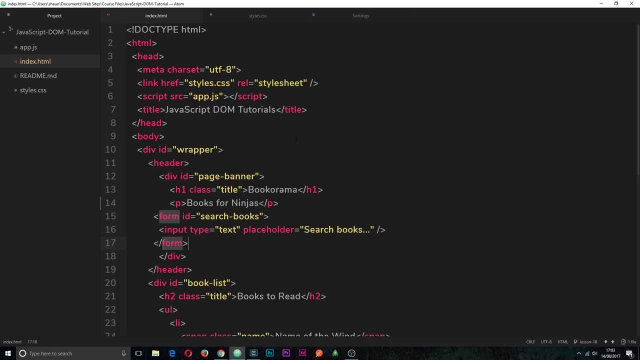 lesson 10 branch, and you're going to see all of that code right here. okay, speaking of code, i'm going to walk you through the html that i've created for this mini application right here. i'm not going to create this from scratch and you can watch it. this isn't a html course. 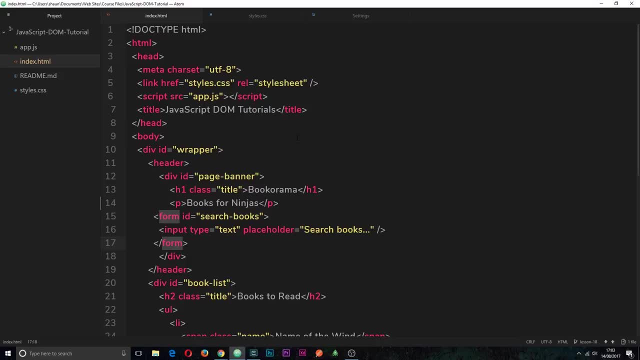 i'm assuming you've already got a base understanding of html, so i'm just going to walk you through it quickly. now in the head, we're just linking up to this style sheet right here which is over there, and i'm going to show you that in a second we have a wrapper down here which is: 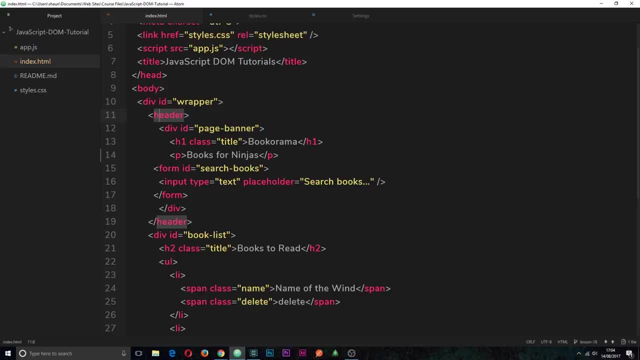 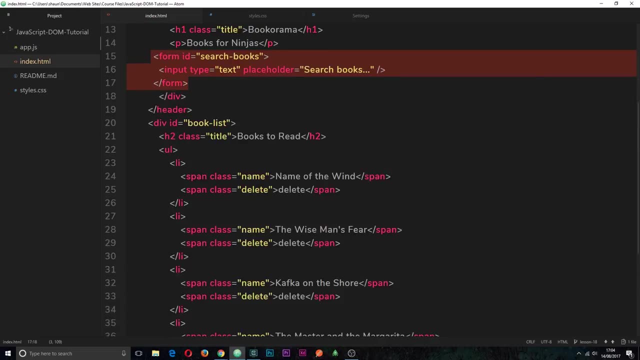 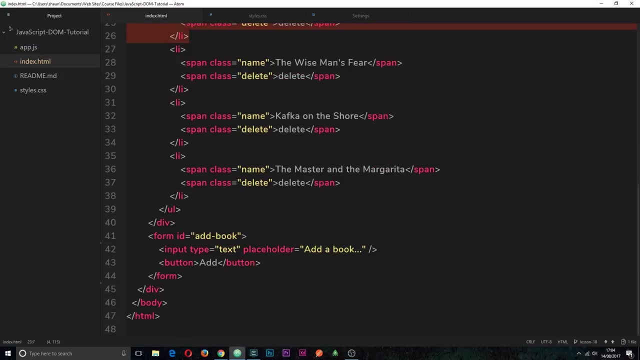 wrapping all of the content, then a header with that form in or round about here. that is for searching for books. we're going to hook up that functionality later on. we also have a div for the book list itself, where every book has its own li tag and below that we have another form to add new. 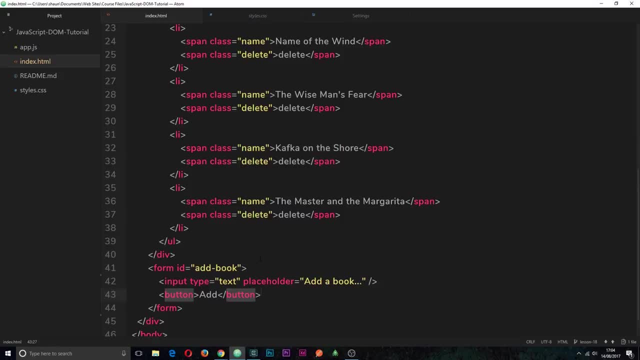 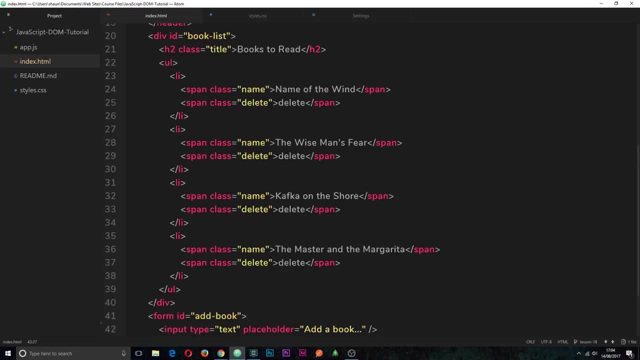 books, which is just an input field and a button. so we're going to add to this as we go along, but this is kind of like the starting point, if you like. so take a look through that, familiarize yourself with it. i'm also going to include this stylescss as the starter files. again, this is not a css course, so i'm not going to 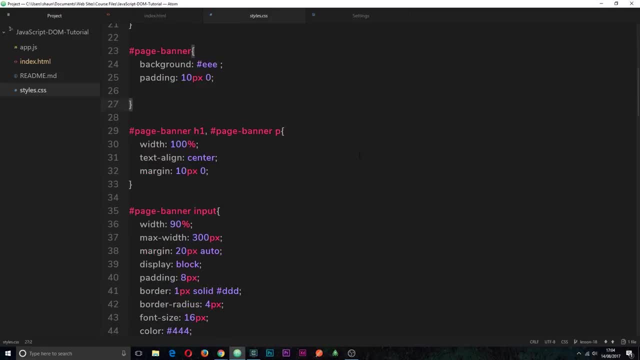 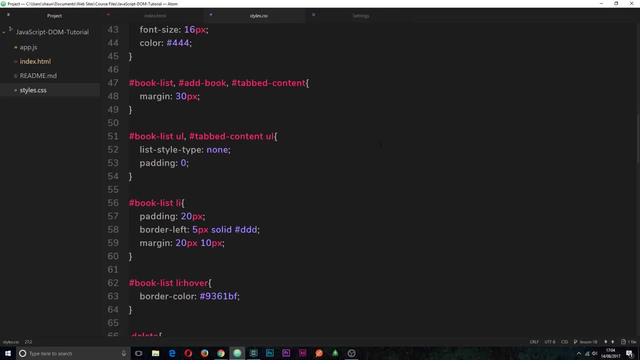 create these from scratch. i see no point. if you want to learn css, i've got a css for beginners tutorial series. i'll leave the link to that down below. but yeah, peruse through these in your own leisure if you wish some really basic styles, just to make it look a little less crappy on the web. 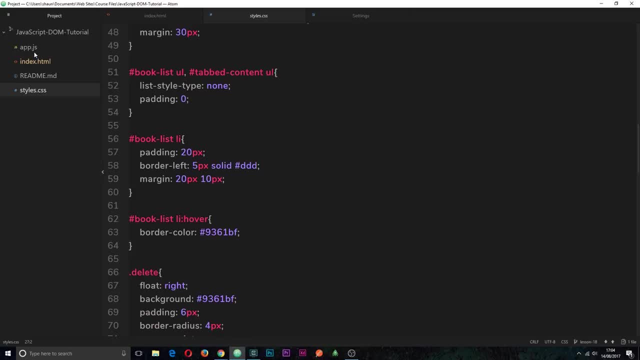 page. all right, we're also going to have this appjs file. that's what we're going to do, all of our javascript as well, and we're going to start on that probably in about two, three lessons time. so that's all for your introduction. if you do like these videos, my friends, please, please, please. 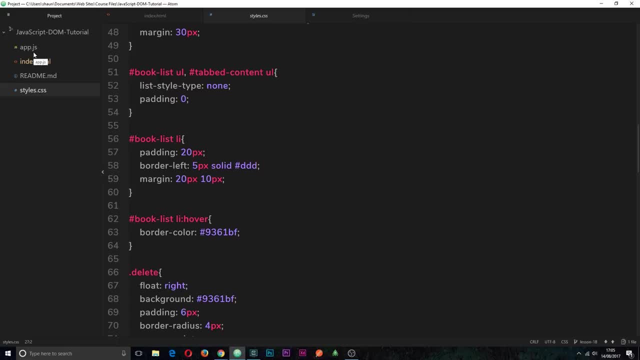 do not forget to like them, subscribe and share them, and i'm going to see you in the very next video. 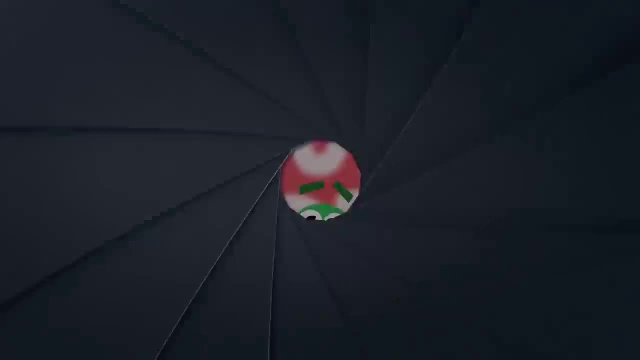 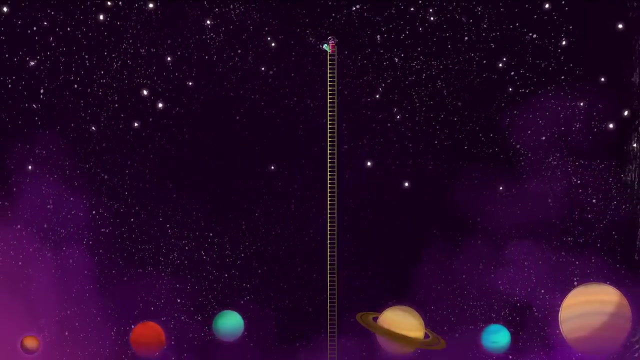 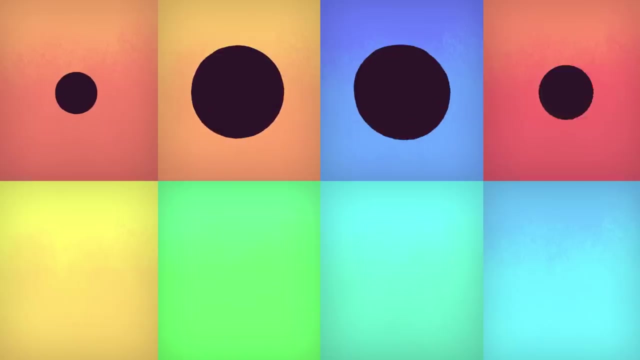 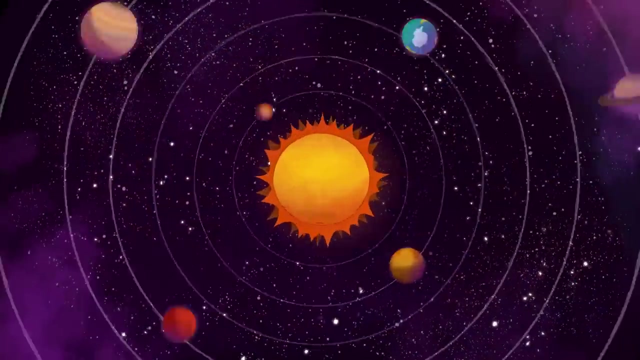 We can see the whole solar system from here. I think we can hear it from here too. We are the planets of the solar system, Different sizes for everyone. The music never ends. We are such good friends And we all orbit the sun. 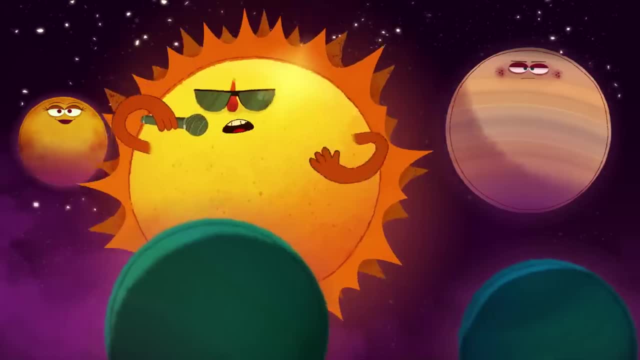 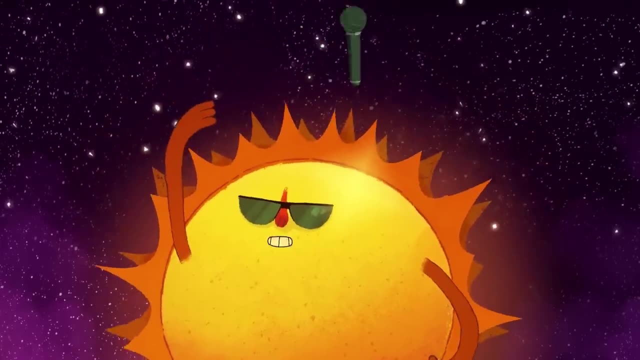 Here comes the sun rapping first on this track. from the beginning, I'm the center of the solar system. Planets be spinning around me So hot I'm roasting. you see, Now I pass the mic to the planet closest to me. 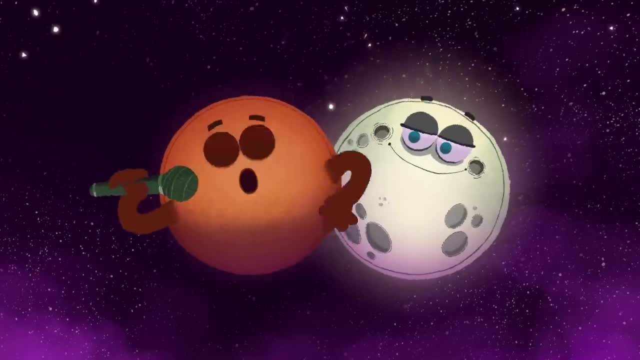 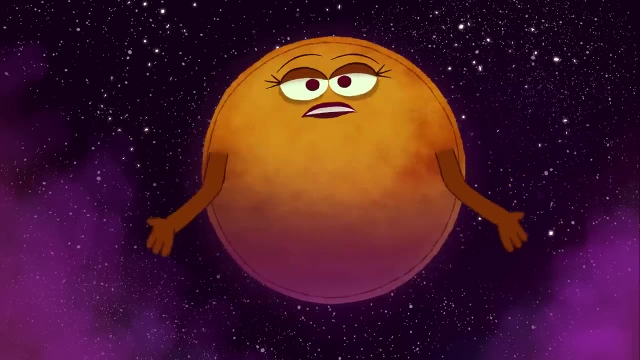 Mercury, the smallest planet, small as Earth's moon. I get super hot and cold and it's been very slow. I'm Venus. I got mountains and volcanoes that spray. I'm the same size as Earth, but spin the opposite way.